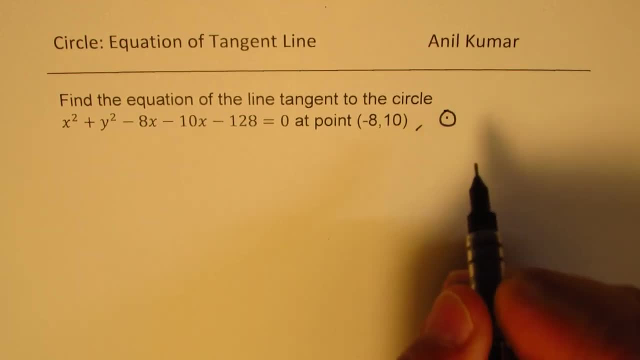 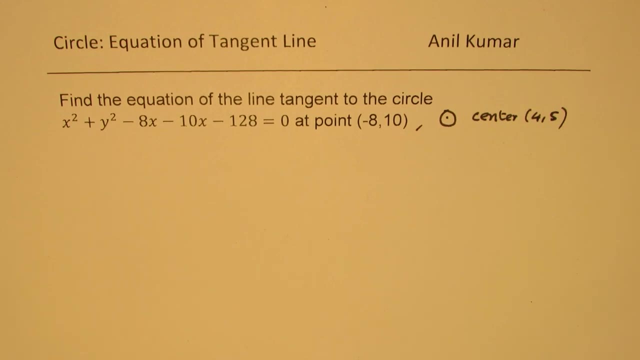 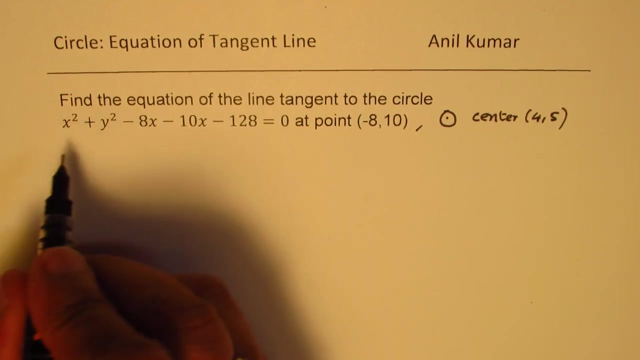 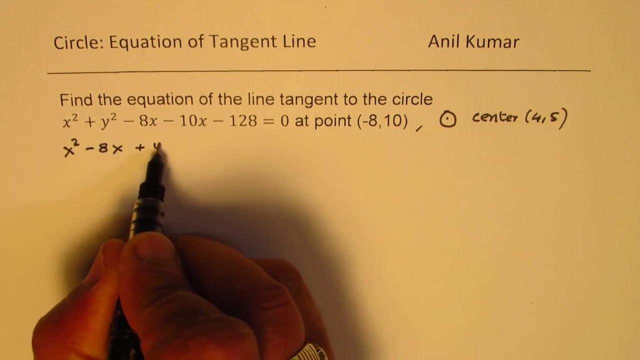 So this is equation of a circle and the center is at 4, 5.. How do we get it? Let me derive this also before we get into equation of tangent line. So we basically do completing the squares. I will just rearrange this equation. We get x square minus 8x, plus y square minus 10y. 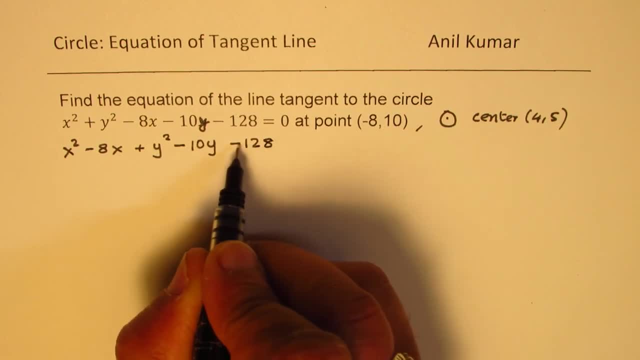 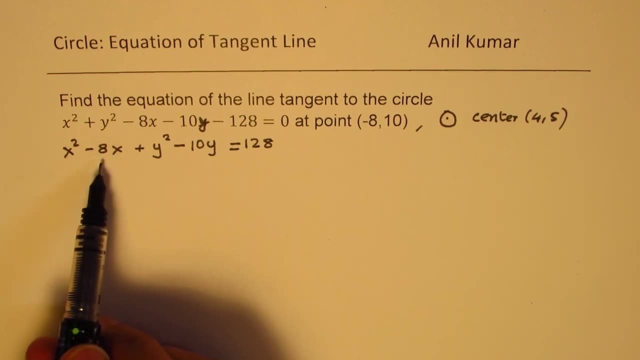 And we have minus 128.. Let me take it to the right side and write it equal to 128.. Now to complete the square, we have to do half of this number, Add and subtract its square, So half of this number is 4.. So we will do x square minus 8x plus 4 square. 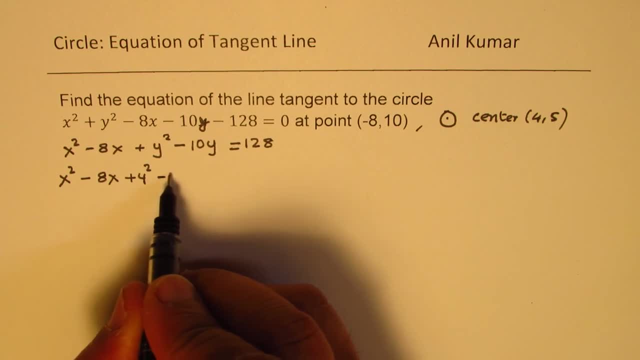 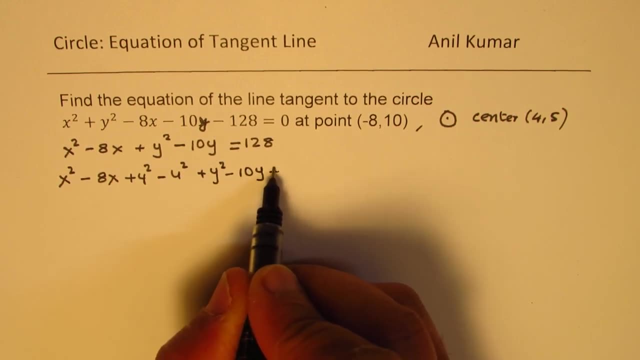 So we can add on the other side also We can write this: minus 4 square here. So plus y square minus 10y plus 5 square, half of 10 minus 5 square. So we are adding and subtracting one number. It doesn't change the equation. 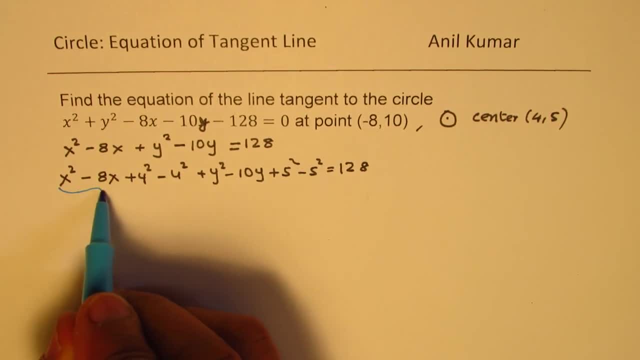 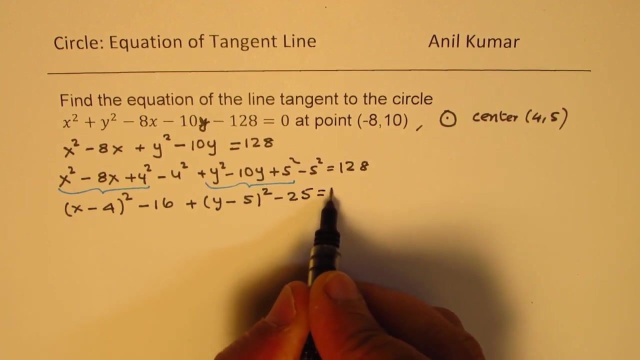 However, doing so, we actually form a perfect square. So these are the perfect squares, and they can be written as x minus 4 whole square, And this is So: we get x minus 16, and then we get plus y minus 5 whole square, and that is minus 25 equals to 128.. 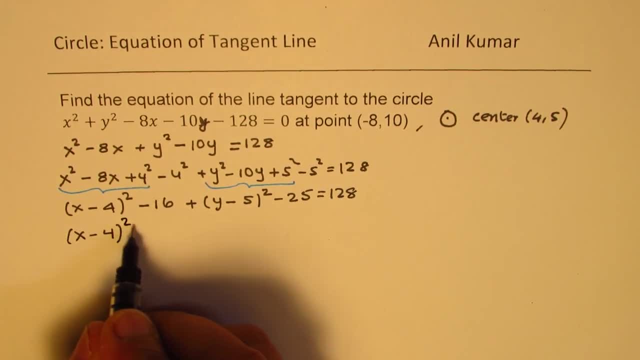 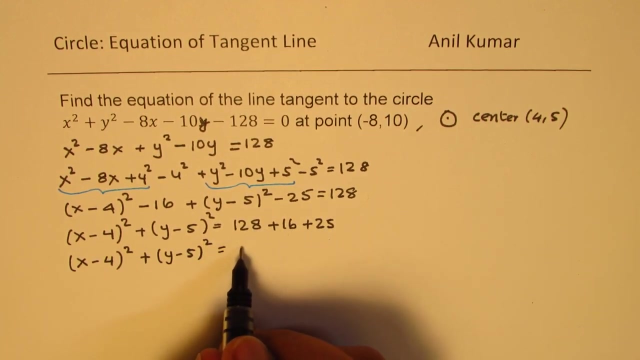 So we get this as x minus 4 whole square plus y minus 5 whole square. Taking these terms to the right, we get 128 plus 16 plus 25.. So we get the equation of circle x minus 4 whole square Plus y minus 4 whole square equals to adding them. we get 169, which is basically 13 square right. 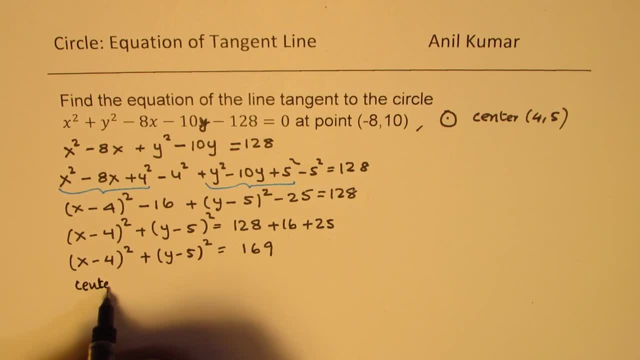 So from here, you know we have the center at the point which is 4 and 5, and we also know radius is 13, right, Since this is equal to 13 square, correct? Now let's get back to our question, which is: find equation of the line tangent to this particular circle. 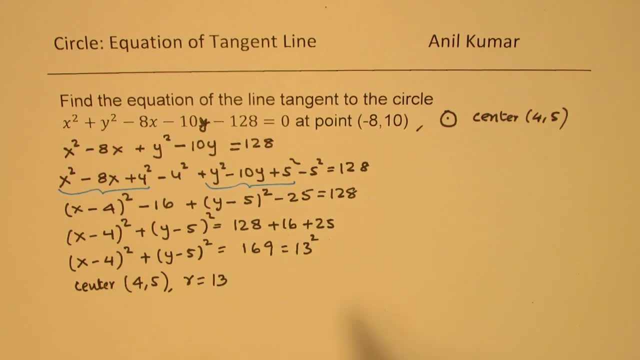 So we know it is a circle. So let me just sketch one here. Okay, Let me make a small sketch. We'll need space to draw, find the solution of the question. So the center is known to us is at 4 and 5.. 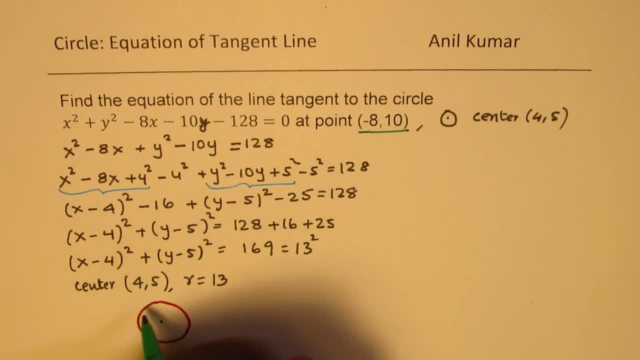 We are looking at a point which is minus 8 and 10.. So definitely somewhere here, And the tangent is kind of like this: Is it okay? The important Thing to realize is that the radius will always be at right angles to the tangent. 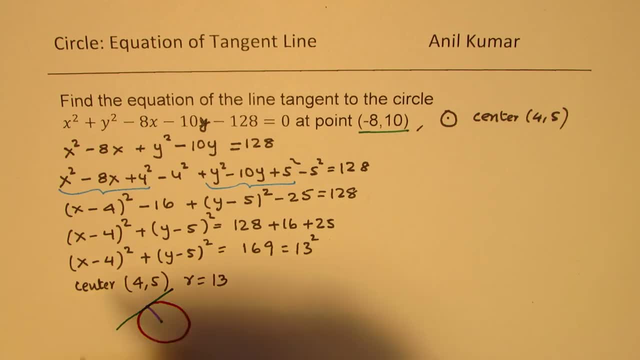 So if I have drawn this radius from the center, it is at right angles. Now, in this particular situation, we know that the center for us is at 4 and 5. So this point is 4 and 5 and that point is minus 8 and 10.. 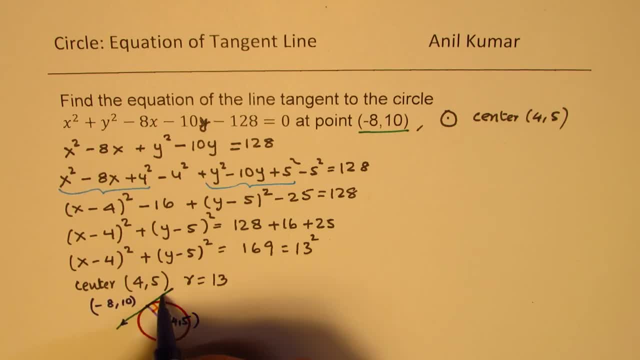 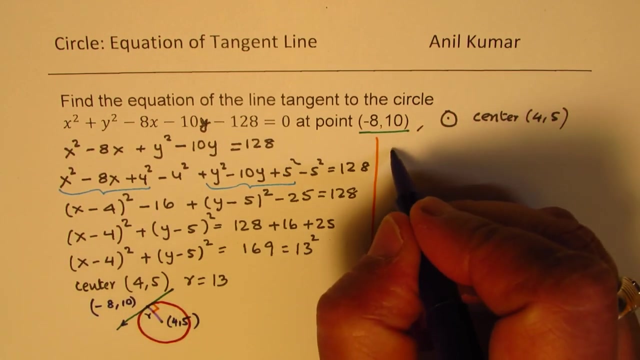 We have to find the equation of this tangent line. Is that clear to you, Right? How do we do that? So the concept is: find the slope of the radius r, Correct? So this is the radius r. So let's find slope m of the radius r. 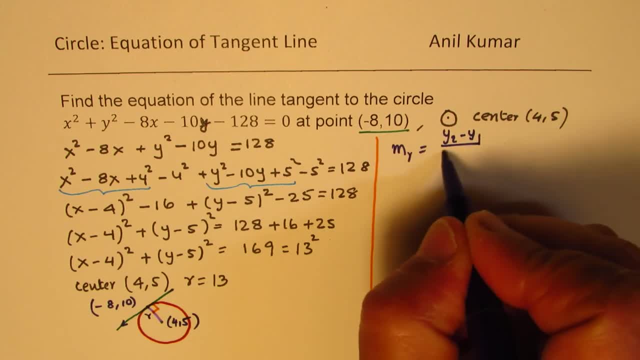 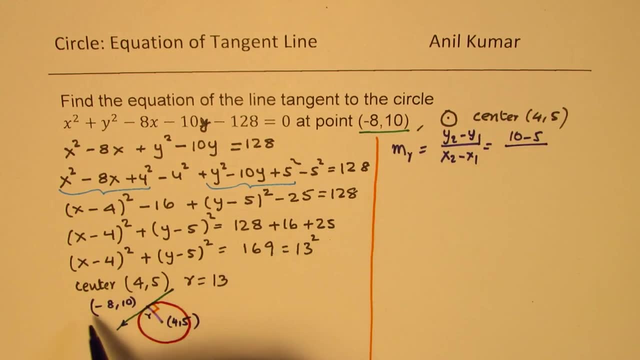 Using the formula y2 minus y1 over x2 minus x1.. Correct, So 10 minus 5.. Over minus 8 minus 4.. Correct, So that gives you 5 over minus 12.. Now for the tangent line. the slope will be perpendicular, right. 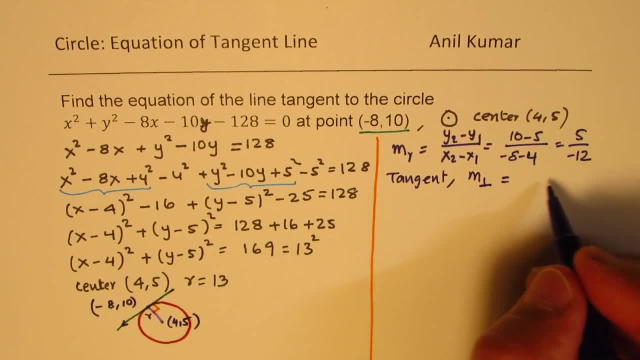 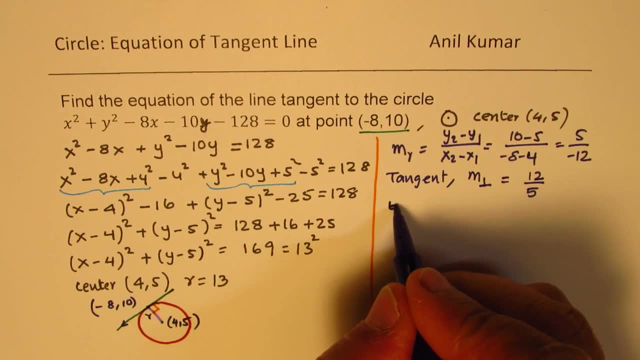 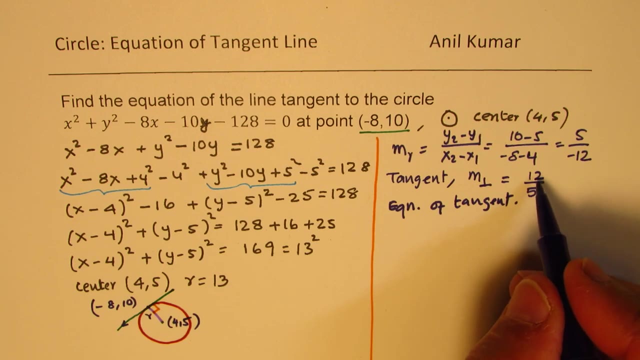 So slope will be perpendicular to this, So that will be negative reciprocal. So it is 12 over 5.. Clear, So now what is the equation of tangent? The equation of tangent will be, We know the slope which is 12 over 5, through the point which is minus 8 and 10.. 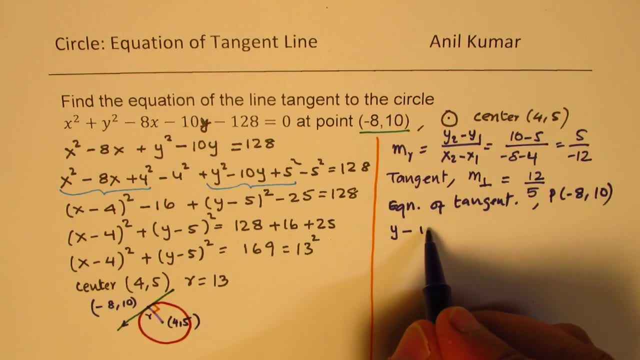 We can use y minus y1, which is 10.. Right Equals to m, which is 12 over 5 times x minus x1, which is now plus 8.. Correct, So that gives you the equation. So what we did here was we use the formula which is y minus y1 is equal to m.